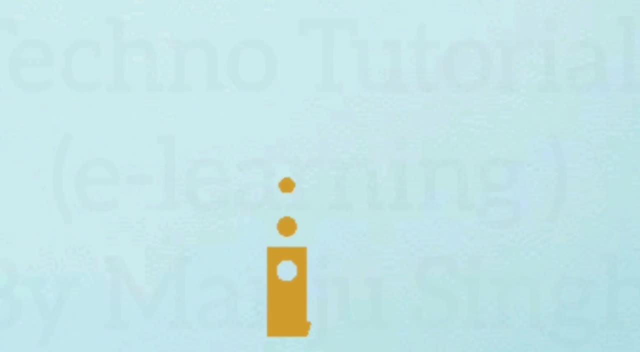 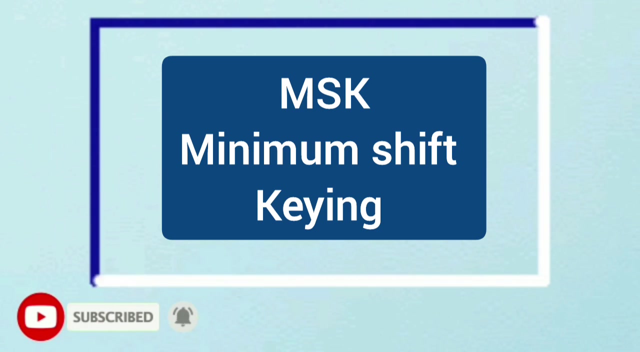 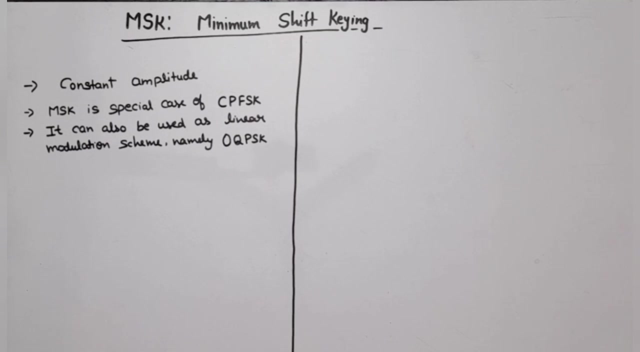 Hello everyone, in this video lecture of digital communication and communication engineering, I am going to discuss MSK. MSK stands for minimum shift keying. So in this video I will. firstly I will discuss the waveform of MSK for a binary bit sequence, then I will discuss 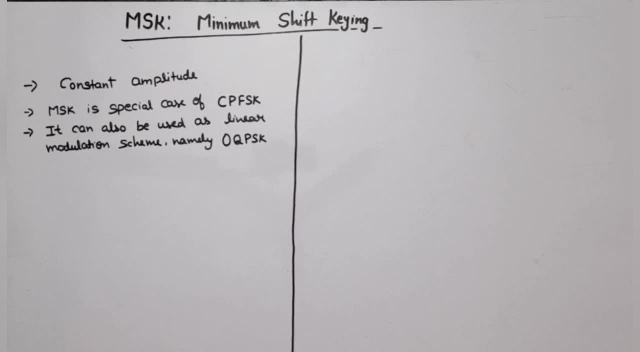 its transmitter, then receiver, then constellation diagram for MSK. after that I will discuss bandwidth of MSK and last I will discuss probability of error for MSK. This modulation technique can be used for linear and non-linear modulation scheme, And in case of MSK, amplitude is constant. 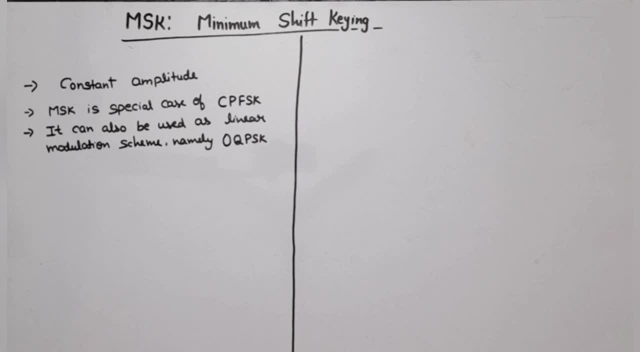 and in case of MSK, there is no adaptive change in amplitude, which was there in QPSK when we were trying to translate symbols Means. this is a special case of CPFSK. CPFSK stands for continuous phase, frequency shift keying. Now frequency shift phase. you told that it will be continuous and in frequency. 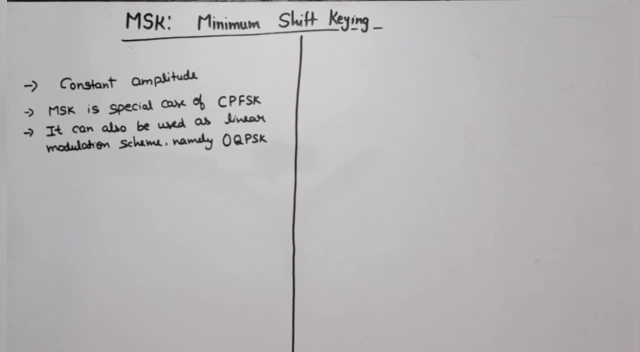 the changes will be very minor changes, very small changes. that's why this is called minimum shift keying And CPFSK. this is the example of non-linear modulation scheme, So in case of MSK we can characterize it as linear modulation scheme as well. in that case, this is called. 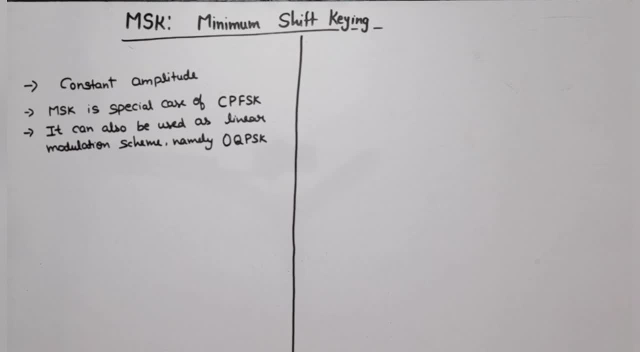 offset, QPSK offset, quadrature, phase shift keying. Now in this: if there are no changes in amplitude, then obviously the probability of error will be good. MSK is used in GSM. in case of MSK, phase is continuous if phase is continuous. that's why what will happen? that there is no inter-symbol. 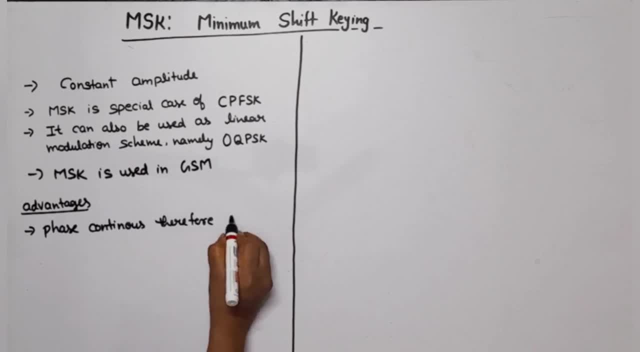 interference. we will multiply the bits with smooth carrier. that's why second advantage is no abrupt change in output wave. now, first of all, we will see its waveform. we will take the sequence 1, 1, triple 0, triple, 1. you can take anything. now we will start its waveform first of all. we will do this. 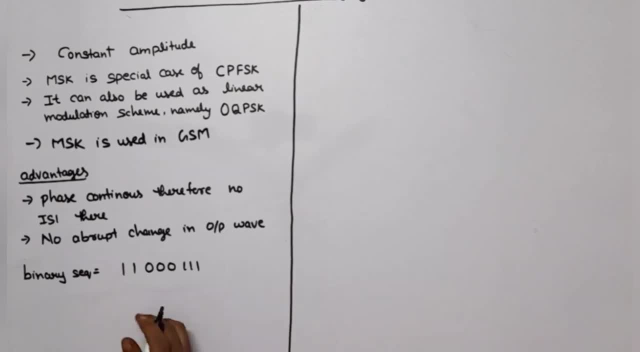 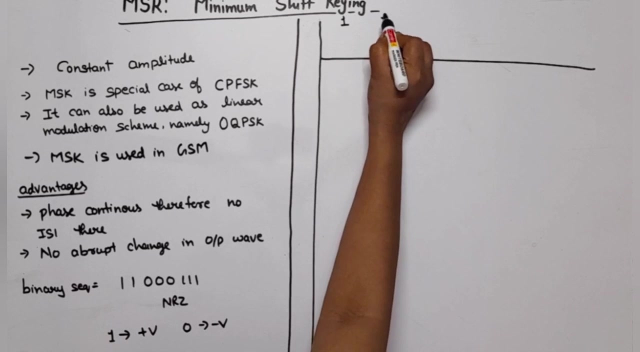 in form of pulses. so for this we will use line coding. line coding, we will use energy technique. energy technique. in that case, we will show 1 with plus V and 0 will show with minus V. ok, what is our sequence? 1, 1, 0, 0, 0, 1, 1, 1. ok, 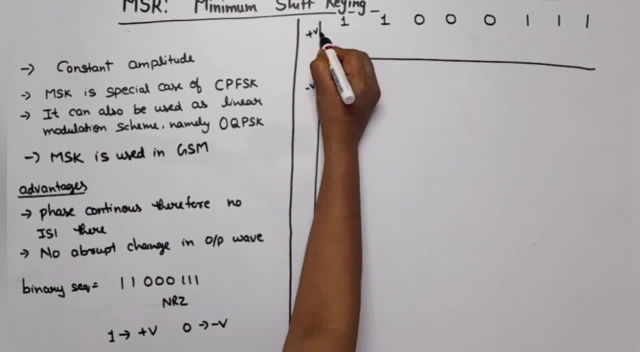 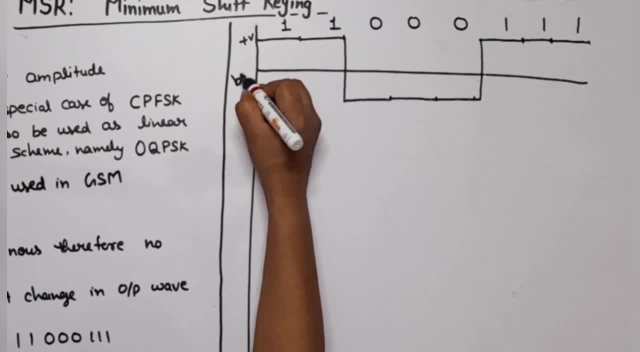 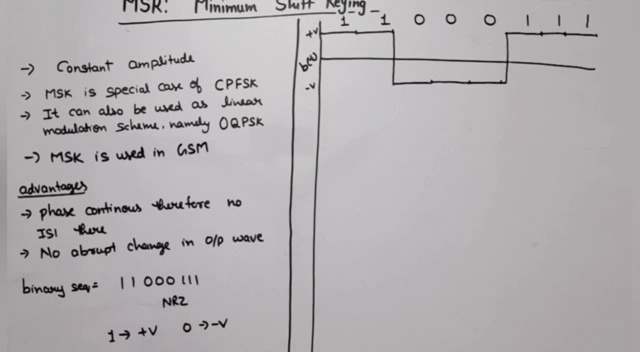 then 1 and then 1. so this is our what happened. this is BT. now we will separate these bits, odd bits and even bits. now we will start the numbering of odd. even our number is this what will happen? 1, 2, 3, 4, 5, 6, 7, 8 means that which our odd bits is. 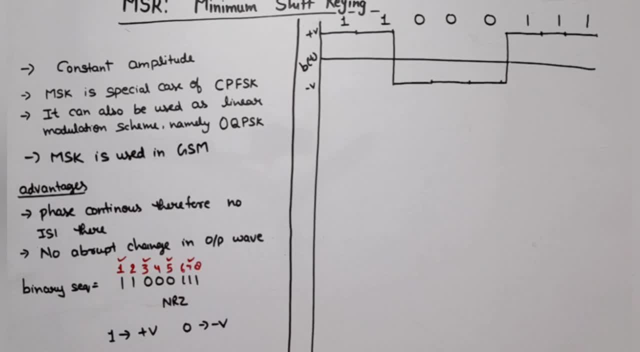 that which is 1, 3, 5, 7. ok, so now, if we now represent these odd bit string, ok, first we take this means tb duration. one bit duration should be same for all bit. ok, now if we divide this in odd, and even If we divide in even, then what will be our B odd T? 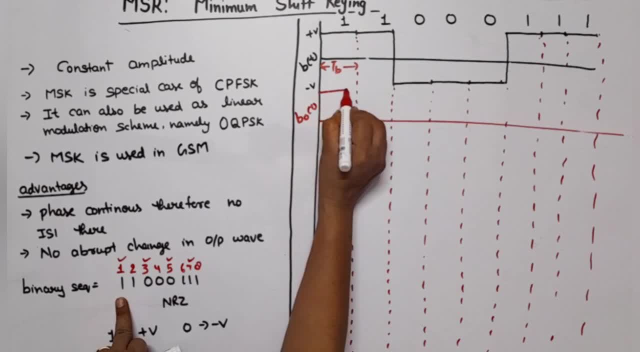 First bit means 1, this is 1, it is odd. Next bit is even. so when will we go to even? We will go to next odd. Next odd is 0, means it will be on 1 for 2 bit duration. 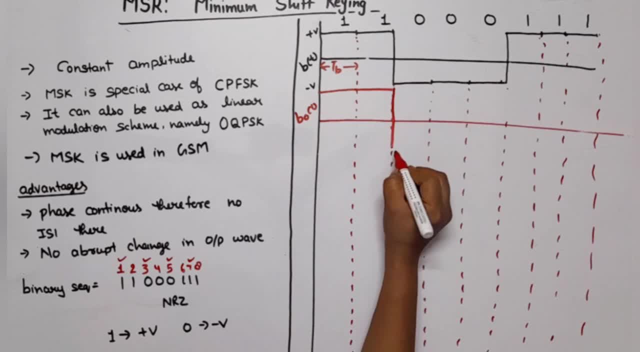 Then 0 means 0, third bit is 0, so it will take 2 bit duration. Then next 0 again, so it will be on 0 for 2 bit duration. Why 2 bit duration? Because even bit is being transmitted separately. 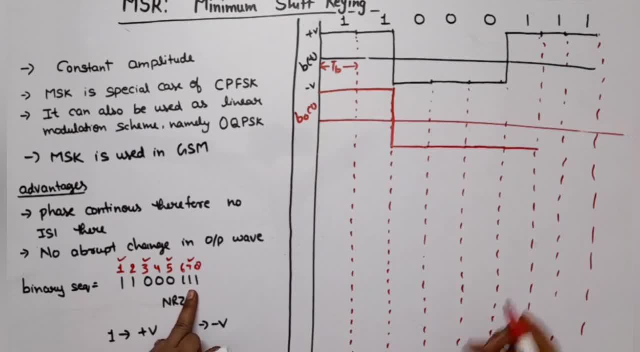 Now next odd bit is 7th bit. on 7th bit we have 1.. 1 means this and it will be for 2 bit duration. This is bit 1, this is bit 3, this is bit 5 and this is bit 7.. 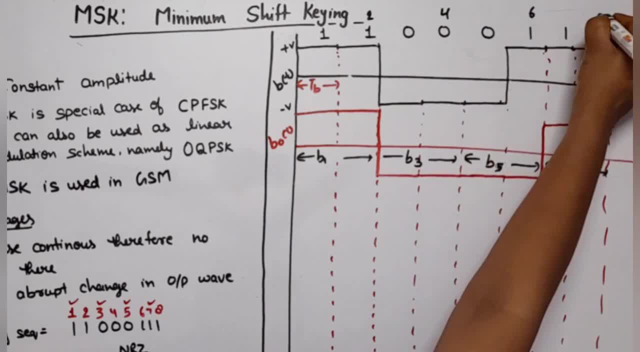 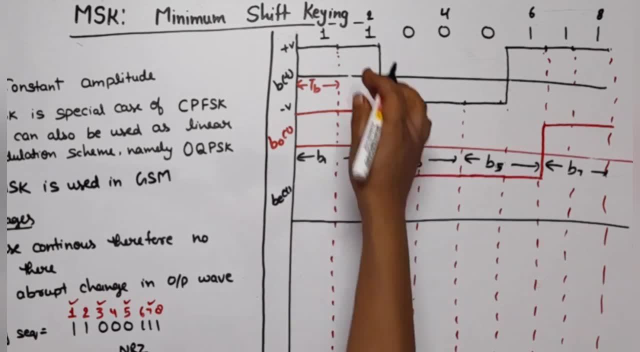 For even we have 2,, 4,, 6 and 8.. But now our even bit is starting from second, so we will write bit even T It is starting from second. what is its value? It is 1.. 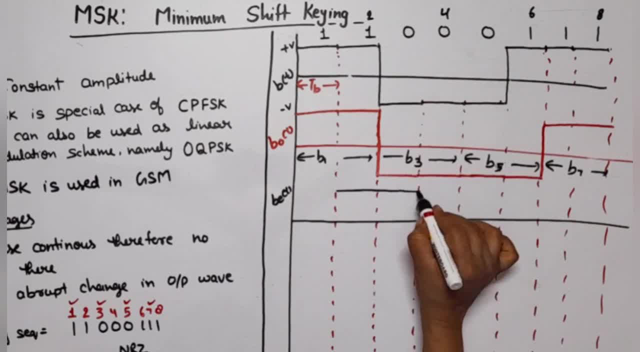 It will be on 1 for 2 bit duration. Then what is on 4th bit: 0.. Next even bit is 0, means for 2 bit duration, 0.. Next 6th bit is 1, means for 2 bit duration, 1.. 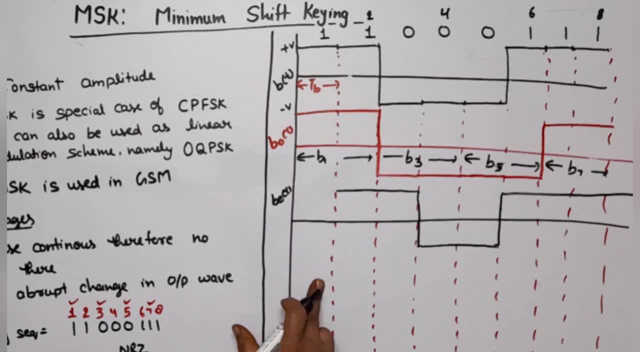 Next 8th bit is 1, means it will be 1 for 2 bit duration. We have separated odd and even. What did we do? first We represented binary bit in the form of pulse. After that we separated both odd bit pulses and even bit pulses. 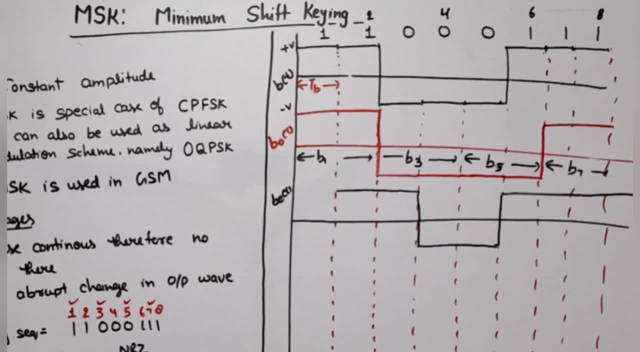 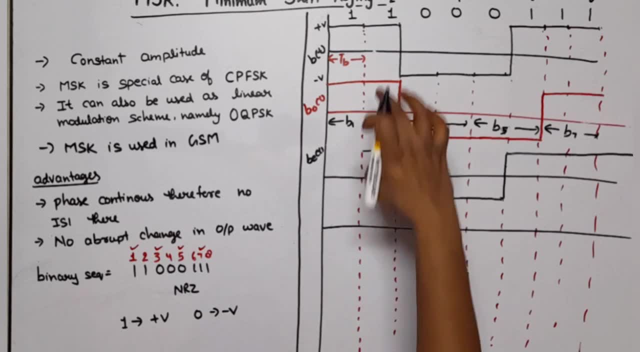 We will multiply even and odd with cos and sin. So we will multiply odd with cos and even with sin. We will show the multiplication of both the bit in this duration. So when we show sin, then how it will be: sin 2 by T by 4TB. 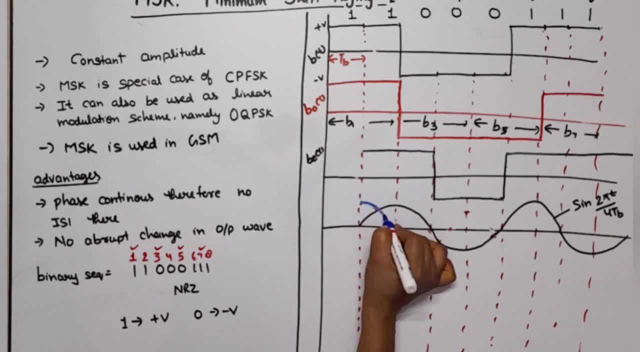 Now we need cos, So we will represent cos. ok, this will be our blue cos. what will be its value? this will be our cos: 2 pi t divided by 4 tb. ok, now we will multiply odd with cos and even will multiply with sine wave. 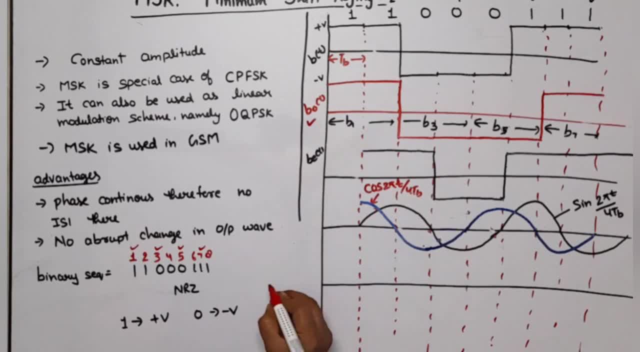 there. what we are going to draw, that is multiplication of this one, and this means that this is b odd t cos 2 pi t divided by 4 tb. ok, now here. what is our first pulse? what is 1 for 2 bit duration. this is our half. means what will be before this. it will go from 0 to here. means: 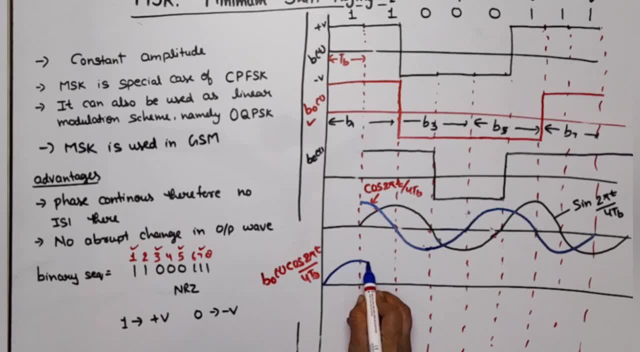 when we draw, then what will be our? this is 1 means 1. ok, now, this is 1. next our odd bit: what is this minus? this minus will be multiplied with this minus. so what will we get? positive, ok, now. next. next odd bit. what is our? again minus 2 pi t. cos 2 pi t divided by 4 tb- ok, 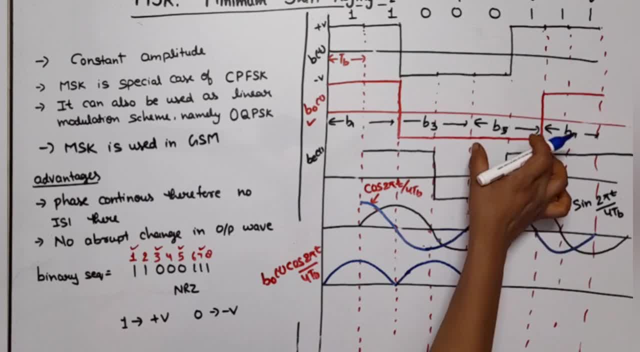 now we multiply it途. see then what will be the same way. and because this 10 meno and this duration also, what is our cos term? so our cos плюс both hersni multiplication is minus. so what we will get is this one. ok, now here. this next bit is 1, and here is same. 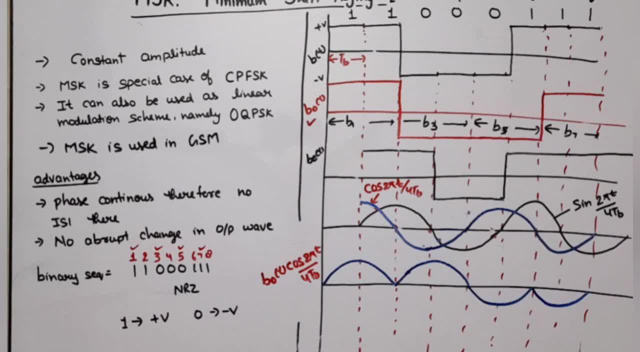 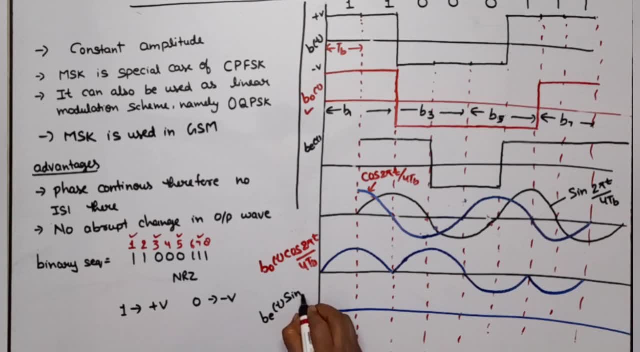 in year, that is minus. now here it means one into minus one, so we will get minus. ok, so after multiplication, here is 3, so 4. now we multiply this even wave with sine. so what? we will get et sine 2 pi t divided by 4 tb. 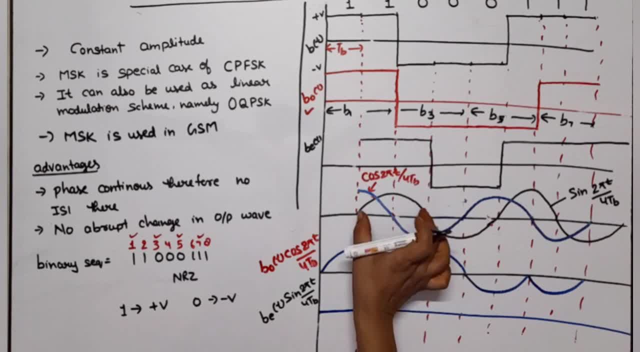 opliない. Now, where do we get our sign from? From here now? sign means that we will observe the black one. positive, positive means for this cycle positive. negative, negative means both are minus, minus. so what will we get? by multiplying Positive- now this is positive. this is positive means positive- now this is positive. this is negative means this will be our negative. so this is the multiplication of this. now we will take two frequencies, carrier frequencies, one of high frequency and one of low frequency. first I take high frequency wave. 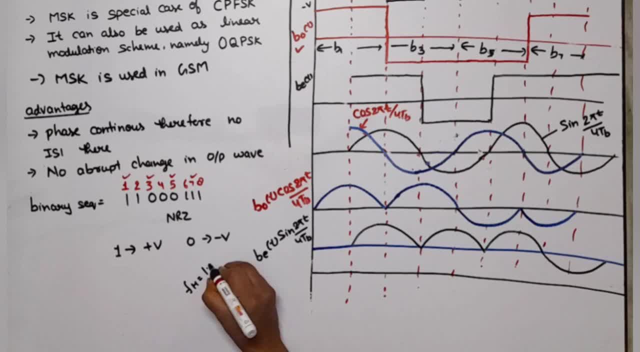 now the difference in the frequency of both of you will be FH, that is, 1.5 FB, and FL will be- that is FB. this is our FL. for this we have taken, FB means 1 bit duration. okay, this is our FL. that is equal to FB. now what we need FH? FH is equal to 1.5, FB means it will be 1.5 times. let's make that okay. 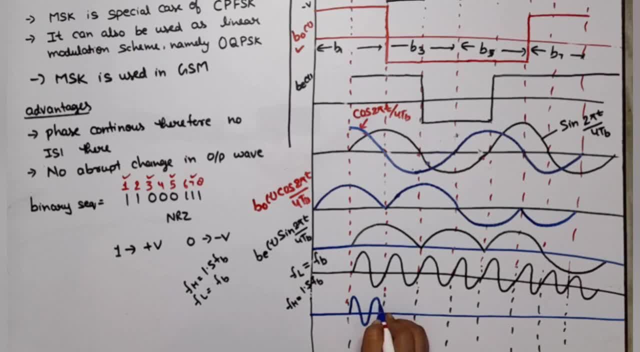 now, what will happen here? 1,, 2,, 3, okay, this is 1.5 times of this. okay, this is our FH and this is our FL. now, now we will get the output of MSK. how will that be? so, in that case, what we will do? we will compare phase of both pulses: if same, then high frequency. if phase is different, then low frequency. 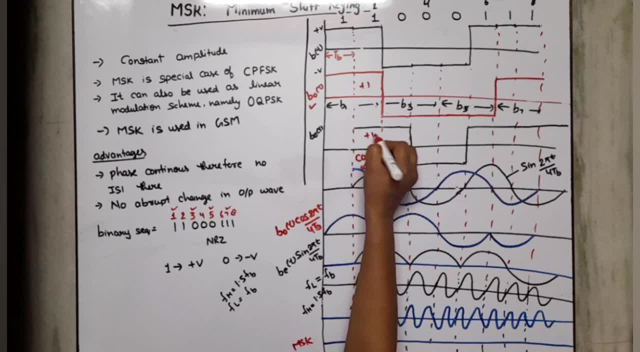 phase of odd and even plus 1, plus 1, minus 1, plus 1, okay, plus 1, plus 1 means same phase, means FH: okay, minus 1, plus 1 means different phase means what will happen. low FL phase will be same phase. phase will not change. 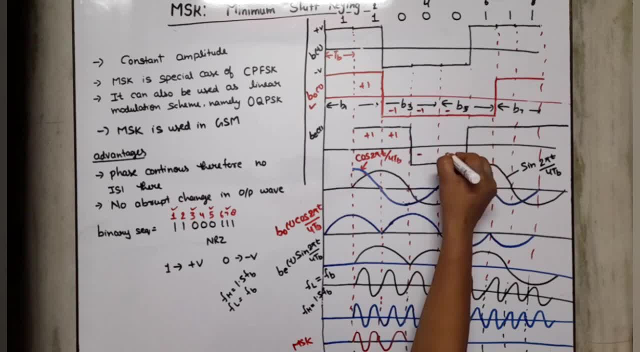 and next, what is here? minus, minus. this is minus, this is minus. okay, this is also minus, minus, this is also minus. minus means both have same phase, means high frequency, okay. next: this is minus, this is plus. means different phase. so what will happen here? low frequency done. next, plus plus, plus, plus, okay. both have plus, plus means high frequency. 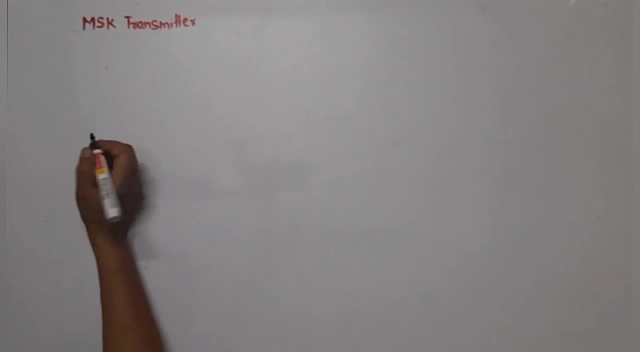 so this is the final MSK wave. okay, MSK transmitter. in case of MSK transmitter on MSK generation, now I am going to draw the block diagram for MSK generation. so in this case, first is what will happen? product modulator: it has two inputs. first input is sin omega CT, that is high frequency wave, and second input is cos. 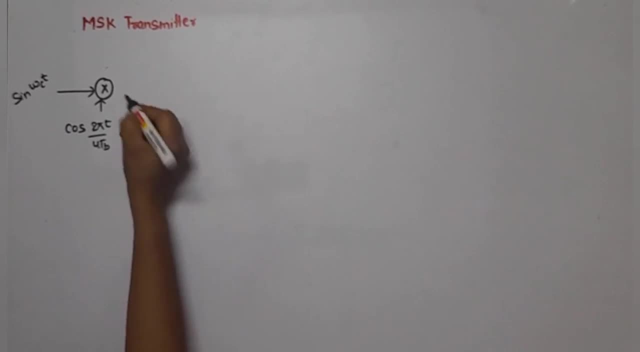 2 pi T by 4 TB, that is low frequency output of this a product modulator. one apply, carrying a, to bend pass filter. first Amara Hoga, bend pass filter 1, and second Mara Amelia, let bend pass filter to the new different frequency per. 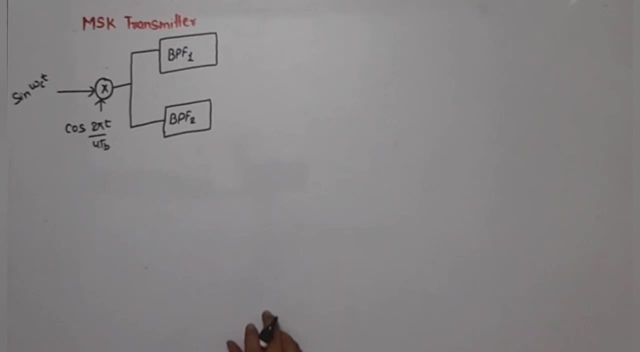 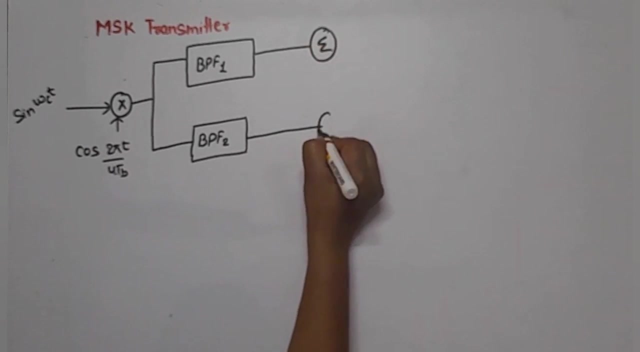 centered only or just for center only us a pass. carrying a. uses Dada. yeah us a comfy frequency co block. carrying a. now I'm can use carrying a one adder and one subtractor. take a, though you have a plus or a plastic, in this case you minus. 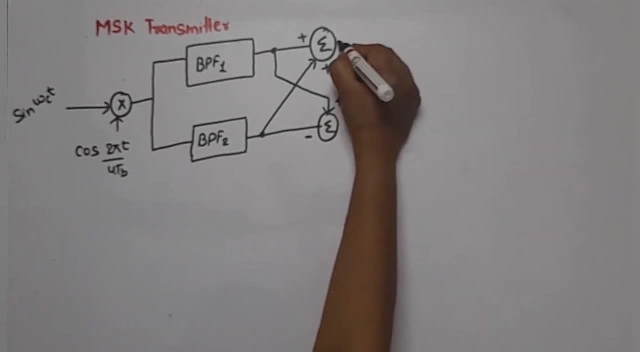 and a plastic and output of these. this adder is applied to one product modulator and subtractor is also applied to product modulator. do you have a product Hoga? you have a Roga odd bit. car means under root 2 PS be odd, P odd bit. 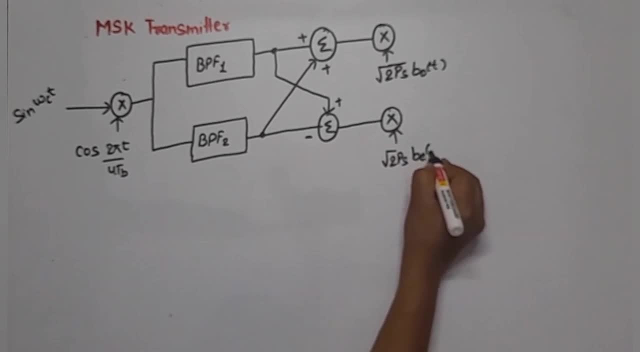 communication. yeah, a multiplication Hoga, even bit car. okay, now output of both product modulator is applied to one more adder. take it: an output of this adder is final m sks. be okay, so your Mari final MSK will be. now agarabi's come at vertical expression. they came to output of this product. 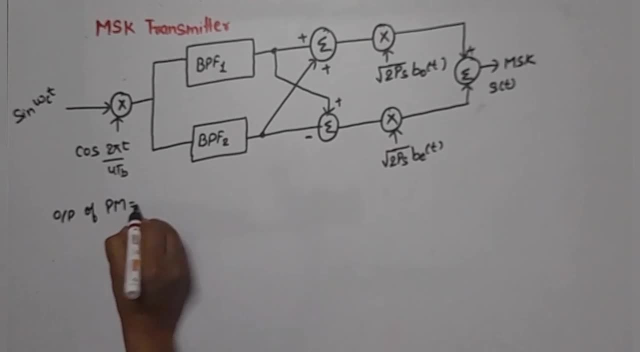 modulator. output of product modulator is equal to sine Omega CT cos 2 pi t by 4 T B. it can be written as 1 by 2 sine a quarter. So it can be written as 1 by 2. sin a means omega c plus b, a plus b means 2 pi by 4 tb. 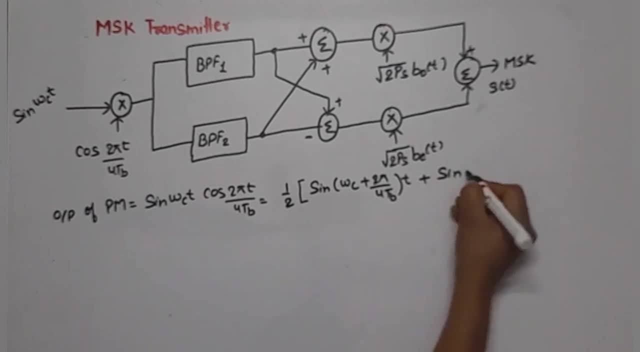 t. then plus sin a minus b means omega c minus 2 pi by 4 tb and t. So now our first band pass filter will be centered on omega c plus 2 pi by 4 tb, and this will be centered on omega c minus 2 pi by 4 tb. output of band pass filter 1 will: 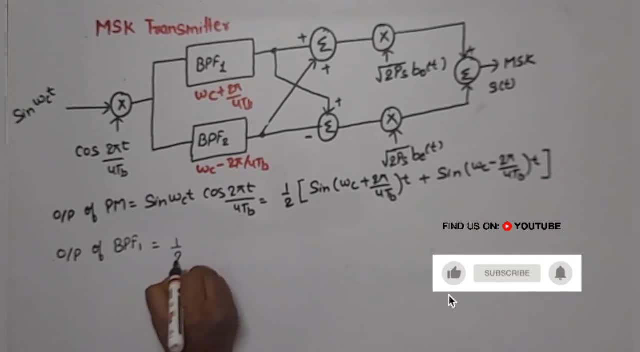 be equal to this will pass. only this will pass. this will block 1 by 2 sin omega c plus 2 pi by 4 tb t. Now output of band pass filter 2. output of band pass filter 2. this is centered at this. 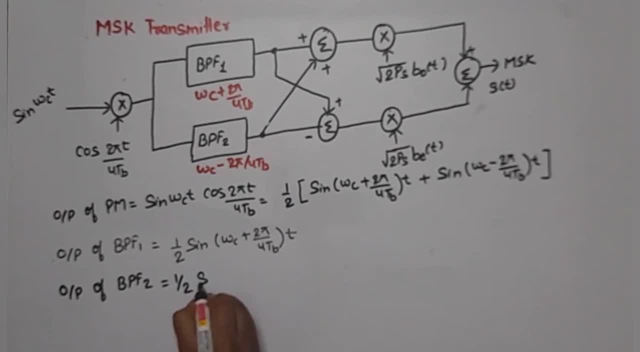 means this will pass. this will block this. So what will happen? 1 by 2 sin omega c minus 2 pi by 4 tb t. Now what we will do? Assume that output of this adder is x1 t and output of subtractor is y1 t. 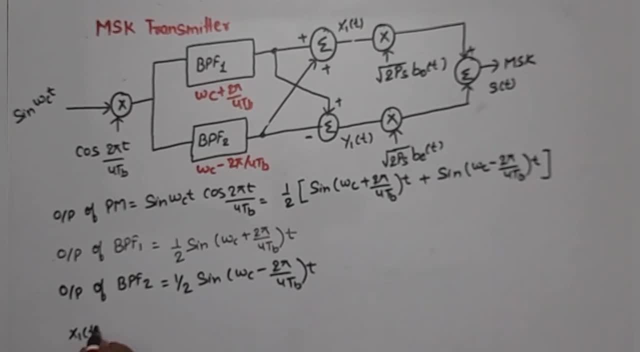 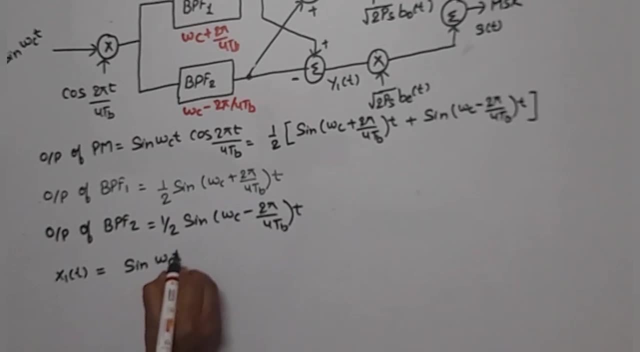 So now, if we write x1, then what will be x1? Summation of these two, this and this which we were getting, this means x1. t will be. that is basically sin, omega c, t, cos, 2, pi, t by 4 tb. 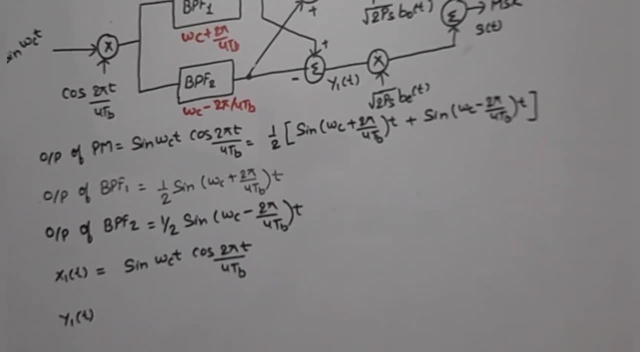 Now what will be y1 t? Now, what will be y1 t? What will be y1 t? Difference will be 1 by 2 sin omega c plus 2 pi, by 4 tb t minus sin omega c minus 2 pi. 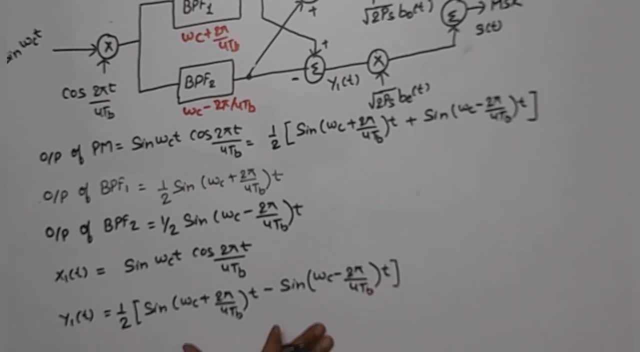 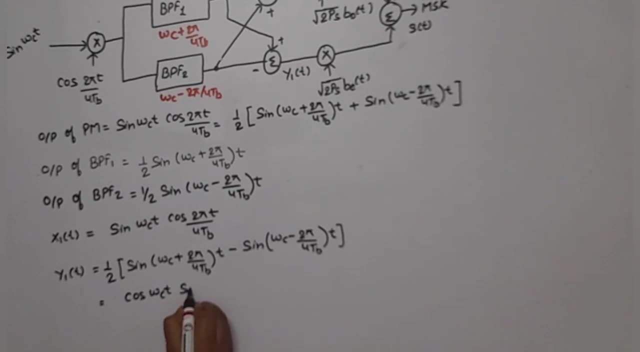 by 4 tb t. So now this formula will be: of whose? This is the formula for cos a sin b. So what will happen? Cos omega c, t sin 2, pi by 4 tb. Okay, Now, x1 and x2 multiplied with odd bit and even bit. and after that, what will we do? 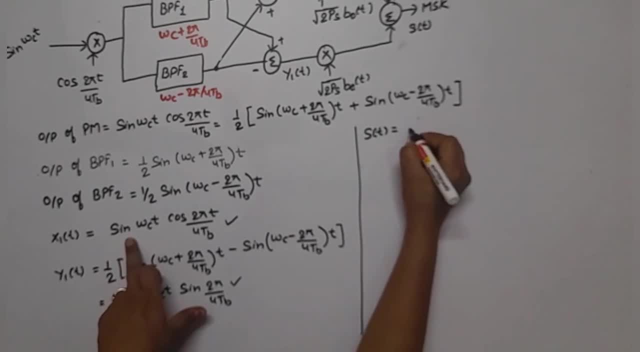 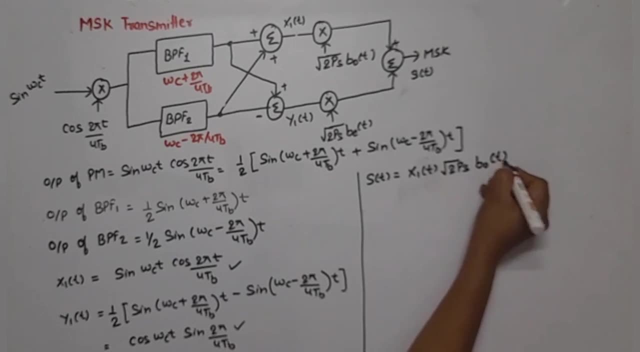 We will add them. So if we multiply with x1 t, what will be our equation? x1 t multiplied with this means under root 2 ps, b, odd t and y1 t multiplied with even bit means under root 2 ps, bit, even t. 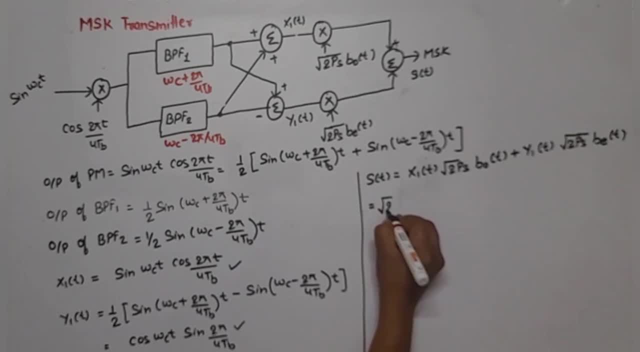 Okay, Now if we put the value of x1 and x2, what can we write Under root? 2 ps bit odd t Sin omega c t cos 2 pi t by 4 tb. And what will happen here? Plus, under root 2 ps bit even t cos omega c t sin 2 pi t by 4 tb. 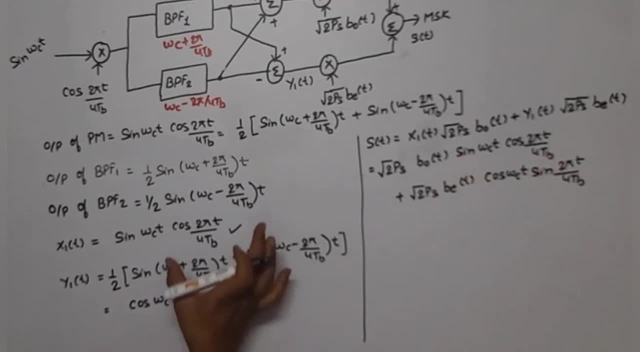 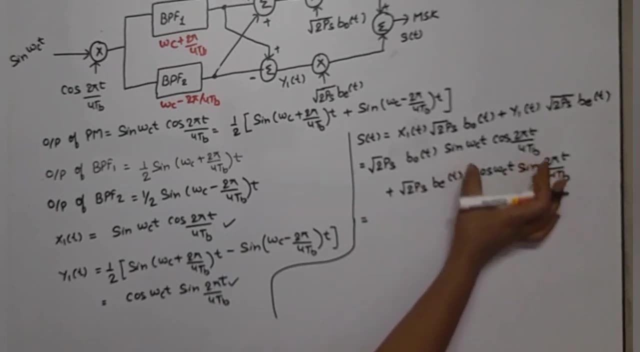 Now, if we expand it, what will be its expansion? This one, Okay. And what will be its expansion? This one, Okay, It will be multiplied with this. So now, if we expand it, what will be the values? 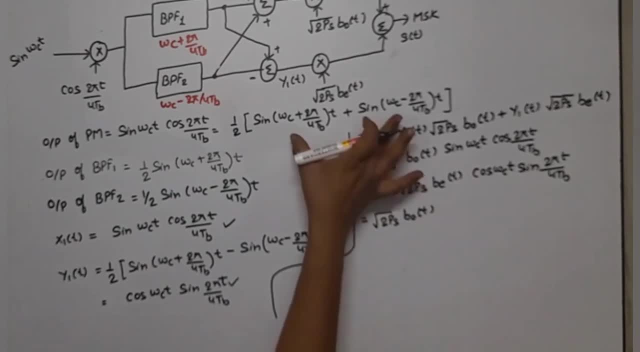 Under root 2 ps. bit odd t. You can directly use it from here And if you want to write, you can write again. What will happen? B naught t. We have expanded this Divided by 2 sin omega c plus 2 pi by 4 tb. 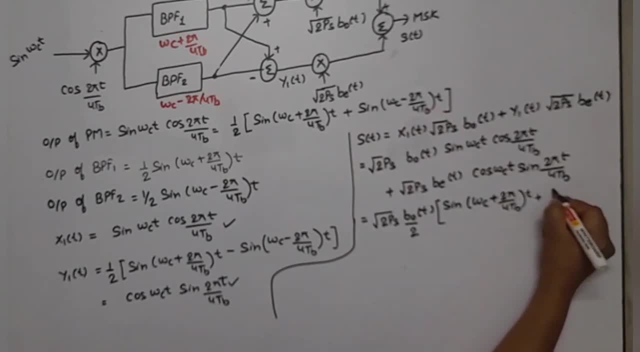 Okay, And the second term will be this: It means plus sin omega c minus 2 pi by 4 tb. Just come Okay. Same way. now we will write this. Its expansion is this: So here we will write: 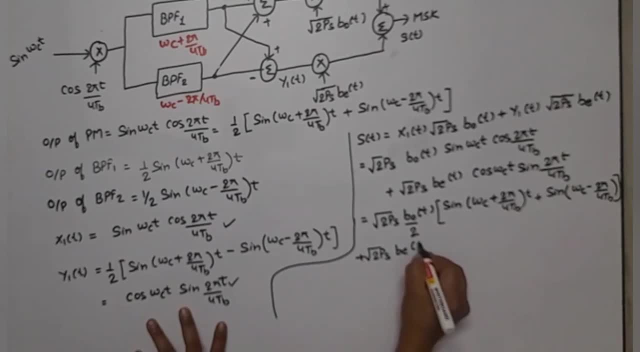 So what will happen? Under root 2 ps bit, even by 2 under bracket sin omega c plus 2 pi by 4 tb And t minus sin omega c minus 2 by 4 tb. Okay, Now we will do these two together and these two together. 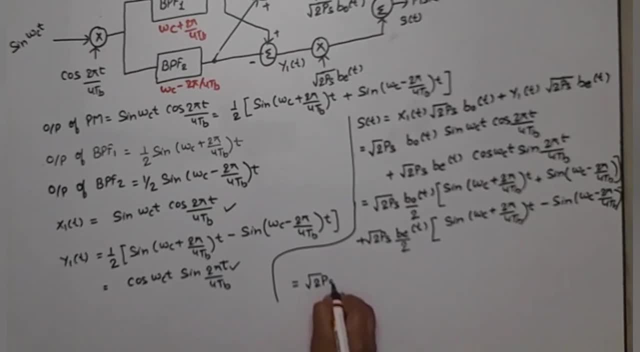 Commonly. In that case what will happen Under root 2 ps? If we take this out, then what will happen? Suppose I took common Sin omega c plus 2 pi by 4 tb t. So what will be the term with this? 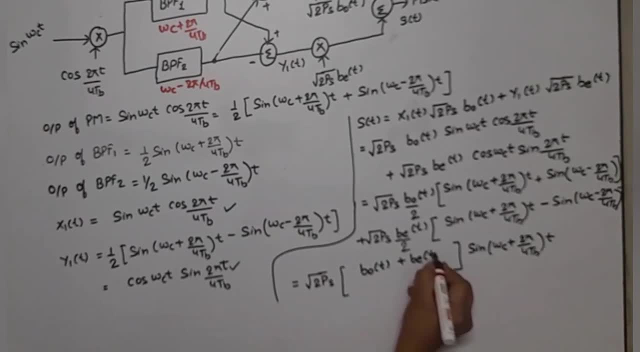 Bit odd t plus bit even t divided by 2.. Okay Now, same way. Now who took? We took minus omega c minus 2.. So here, bit odd minus bit even will come Means. what will be the next term? 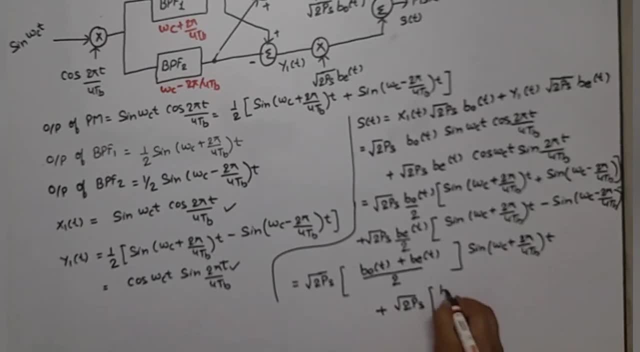 Plus under root 2 ps under bracket bit odd T minus bit even t divided by 2 bracket close sin omega c minus 2 pi by 4 tb and t. Okay, So this is the final equation. Now what will we take? 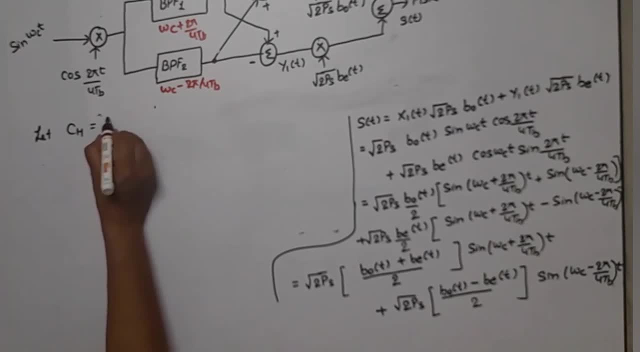 Let ch Where addition is happening. So we have shown this with one variable. So what will happen? Bit odd plus bit even, t divided by 2.. And where minus is happening, We take this Cl. What will happen? 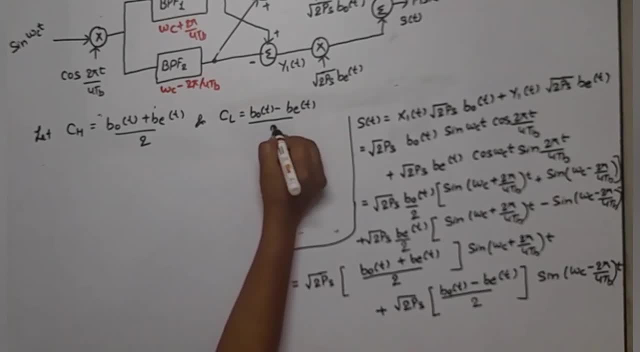 Bit odd t minus bit even t Divided by 2.. Okay, Now let's see the frequencies. Here. high frequency is there Because carrier may be added Here. carrier minus happened. So we take this: Omega h is equal to omega c plus 2 pi by 4 tb. 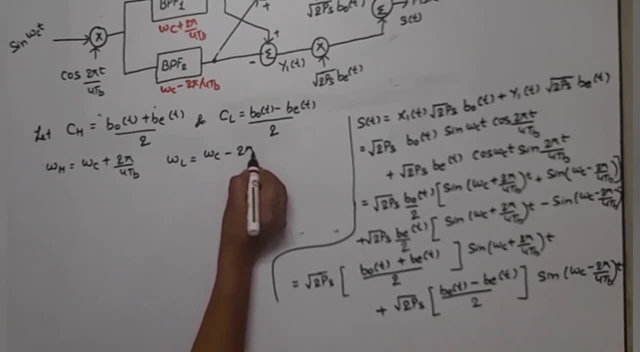 And omega l is equal to omega c minus 2 pi by 4 tb. Now if we take these values, then what will be our equation? Then our equation will be: st is equal to under root 2 ps. This is represented by ch. 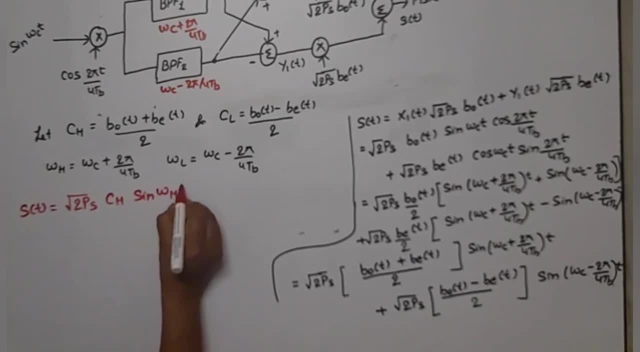 And what will be our sign? Omega h t plus, under root 2 ps cl sine omega l t. Okay, So this is final expression For these two cases. two cases are made. If case 1, what will happen? Case 1.. 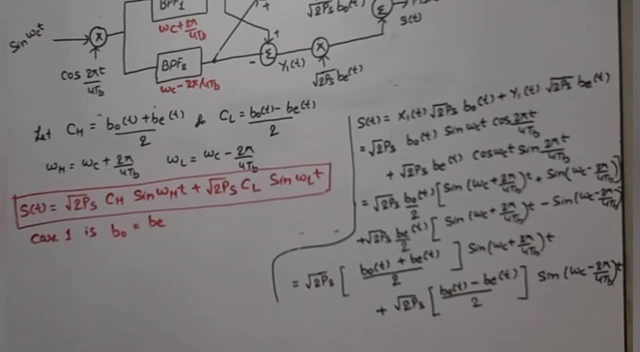 If b odd is equal to bit, even If both are equal, then this value will be. What will be the value of cl Zero? Okay, And if both are plus, then what will happen? Plus 1, plus 1 by 2.. 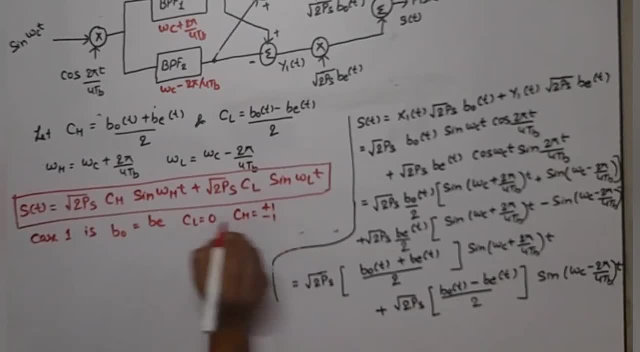 What will happen? What will be the value of ch, Either plus 1 or minus 1.. How, If both are 1, then what will be their amplitude? Plus 1, plus 1 divided by 2.. If both are minus, then what will happen? 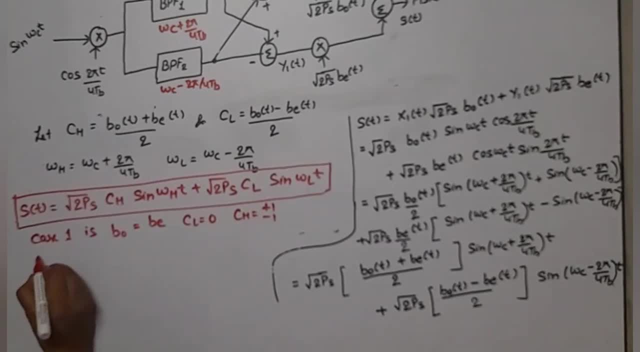 Minus 1, minus 1 divided by 2.. So what will be minus 1?? And case 2, what will happen? Case 2 is if bit odd is equal to minus bit. even In this case, what will happen? 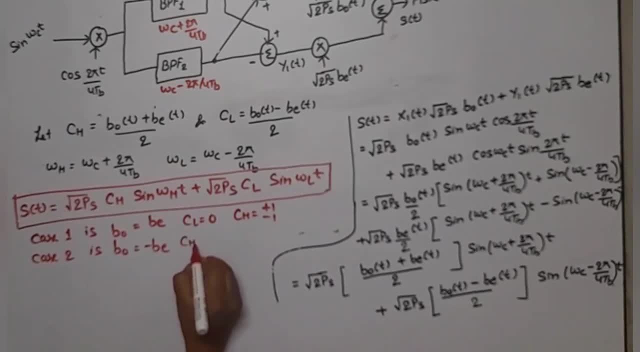 Ch value will be zero. In this case, ch is equal to zero, Because if we have b odd equal to minus b, even then it will become zero. And what will we get in this term? Here we will get: cl is equal to plus 1, minus 1.. 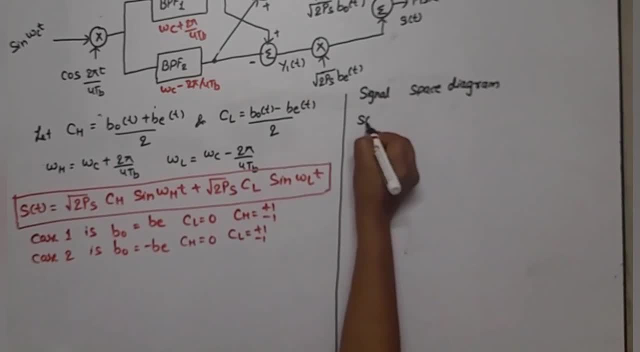 Consolation diagram. So what will happen in this case? What equation do we have? Our equation is st. What we can write this Under root 2ps is ch. If we divide by ts with this and multiply by ts. 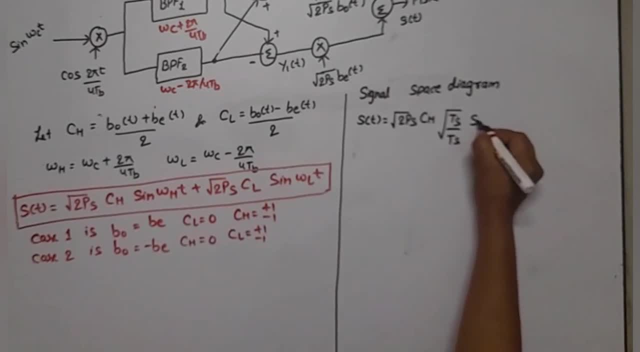 then in that case, if we do this, then what we can write this equation: Sine omega ht plus under root 2, ps cl. here also ts by ts. here what will happen? sin omega L, t. Now rearrange this, So we will take ps ts ch. 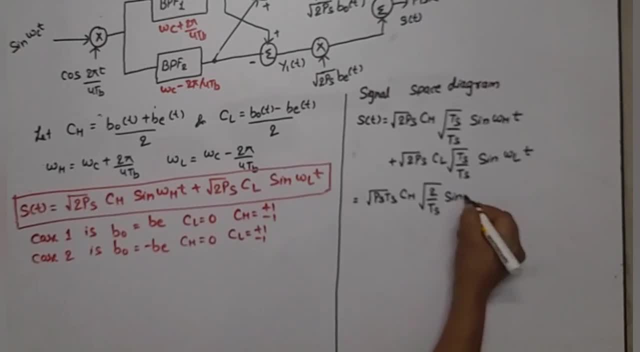 under root 2 by ts sin omega H t. Here it will be plus ps ts cl. under root 2 by ts sin omega L t. Now this is business function phi H and this is business function phi L. Now it can be written as under root. it can be written as es ch. What will happen phi? 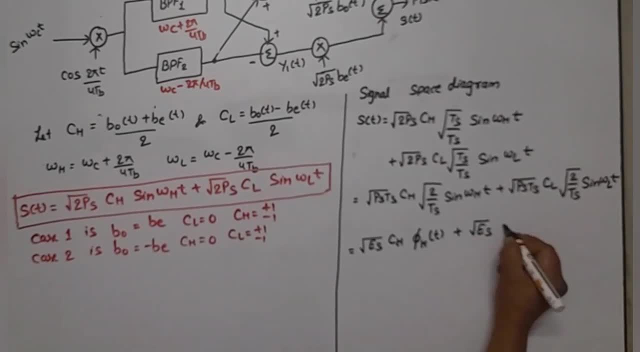 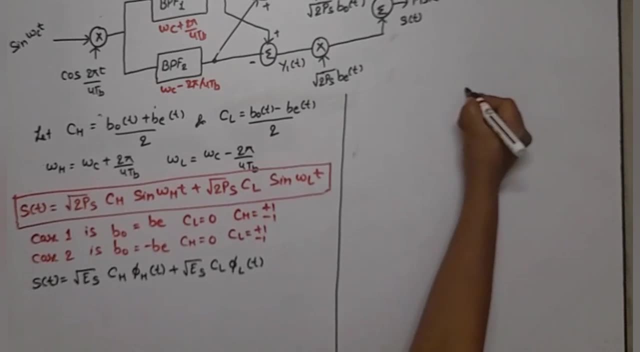 H t plus under root es cl. and what will happen? phi L t. I will write the equation here. Now let us draw its single space diagram. On this axis we took phi H t and here we took phi L t. Now our order will be even bits. What is our coordinate? 1 and 0.. If this 1 and 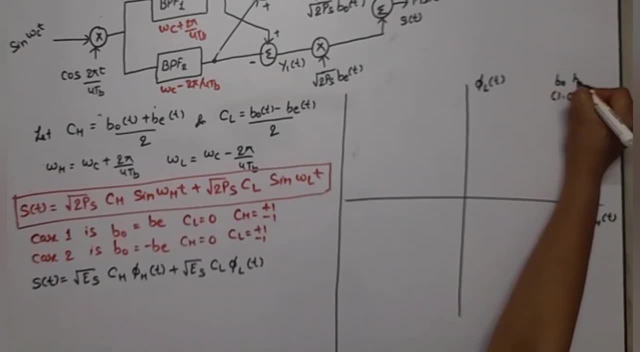 0 is 0,, then what happened? This bit is odd and this bit is even. If bit odd is 1 and bit even is 0, then what will be the amplitude for bit odd, What will be the amplitude for bit odd Plus 1, and what will be the amplitude for bit even Minus 1.. Now, what will be the 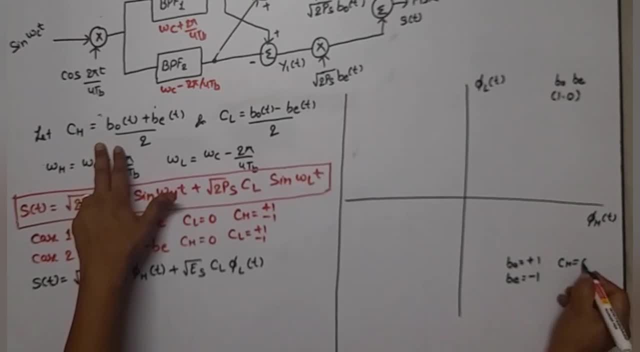 value of ch. If we put the value here, then what will be the value of ch 0 and what will be the value of cl In this case? if we put this value, then 1.. So what was our cl? What? 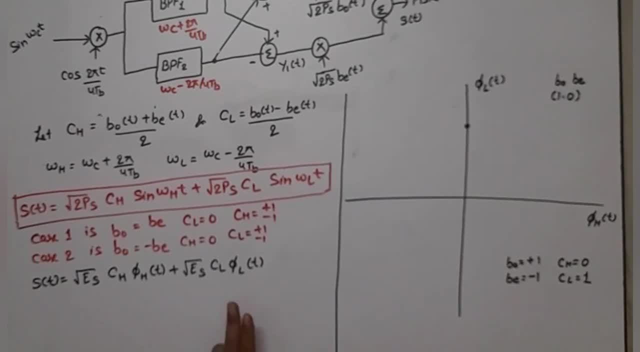 was the value of phi L. Where will we get the point Here Now? in the same way, now it passed through here här and desirable fit that either give it varial value in the descriptor or get 1 and nothing is needed Itatedally. the point must be satisfied here. 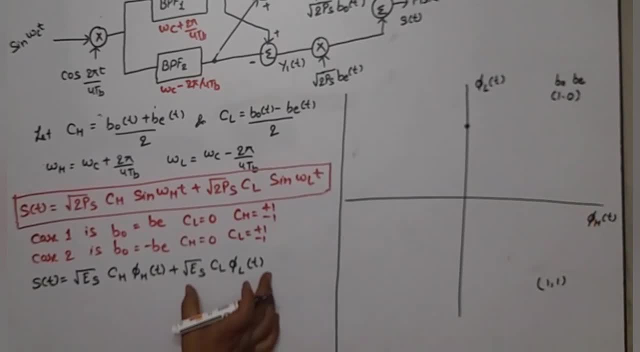 Now what should be the value of ch, of ch? If it is ch, then what do we get? 1 and what is the value of cl? There is a value of ch here to make it possible that we get 0 and 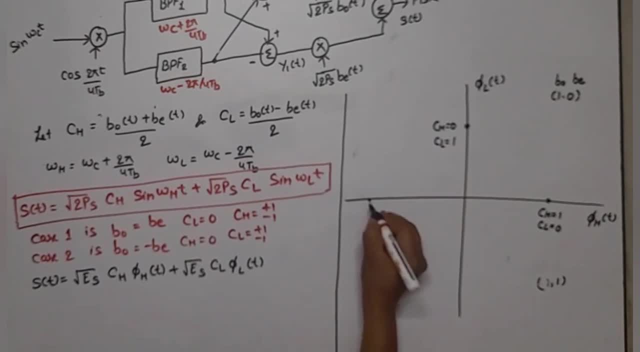 value is 1.. Similarly, our points will be here also. Here the point will be this point 4, 2, 0 and this will be our 4, 0, 1.. So now we will work with two points D minimum. 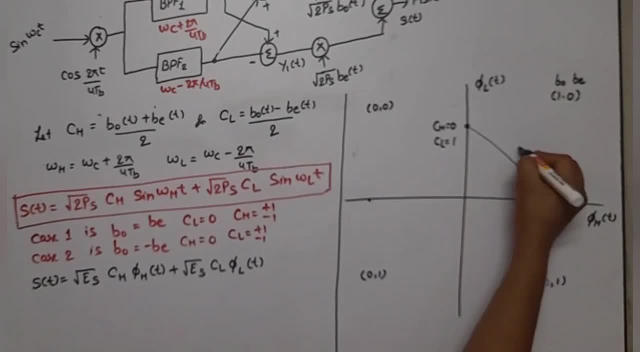 means the distance between these two points. Now, if we have to find its distance, let, this is D minimum. So now this distance, in this term, the value of CH is 0, means this term will be 0,. CL1 means this amplitude. what will happen? Yes, Where This point to? 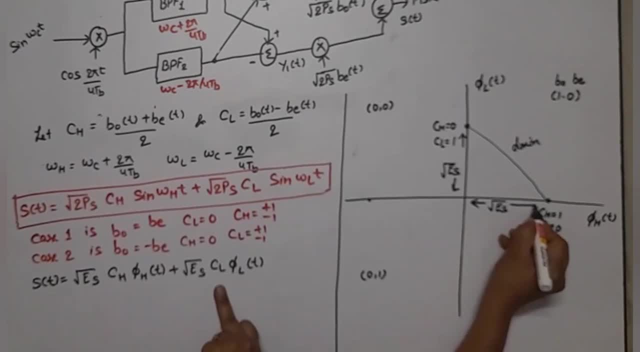 this point. Same way. what will happen here? This is under root ES. Okay, So now D minimum. what will happen? Let us remove here D minimum is equal to under root this square plus this square. So what will happen? ES plus ES is equal to 2 ES. ES is the symbol: energy Symbol. 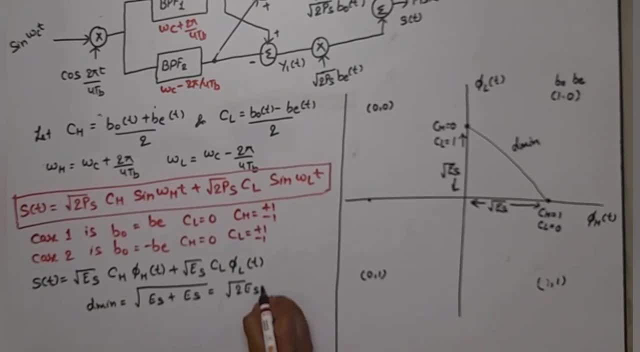 is our 2 bit combination, And if we have to convert in the form of bit, then this will be equal to 2 into 2 EB. Okay, So what will happen? D minimum is equal to 2 under root EB. 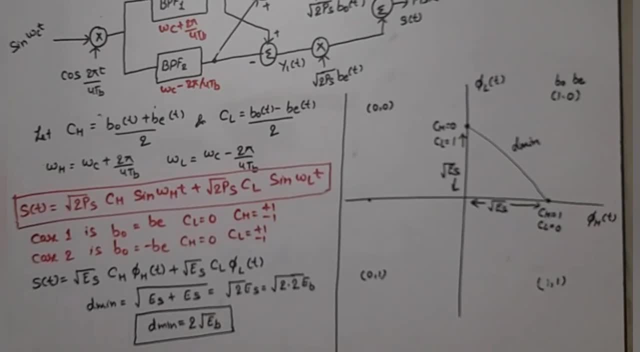 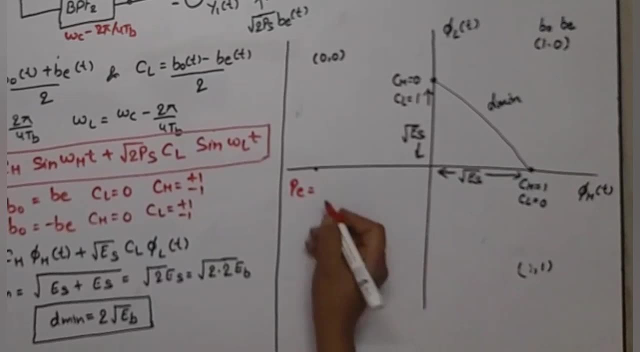 Okay. Okay, This is the consolation diagram and this is the D minimum. Now we know D minimum, So let us remove probability of error. Probability of error is given by 1 by 2. complementary error function, D minimum divided by 2 under root eta. Okay, This is the formula for probability. 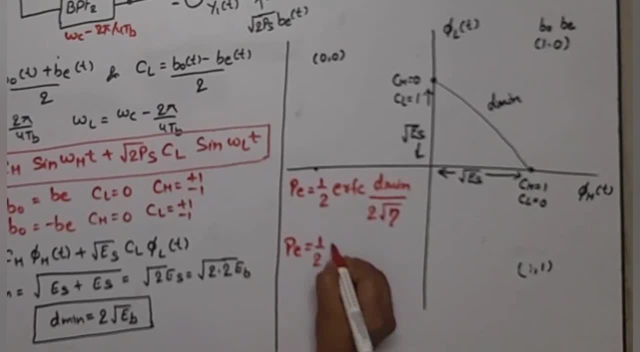 of error. So if we put the value here, then PE will be equal to 1 by 2 ERFC. D minimum is 2 under root. EB divided by 2 under root eta is equal to 1 by 2 ERFC. So this is the. 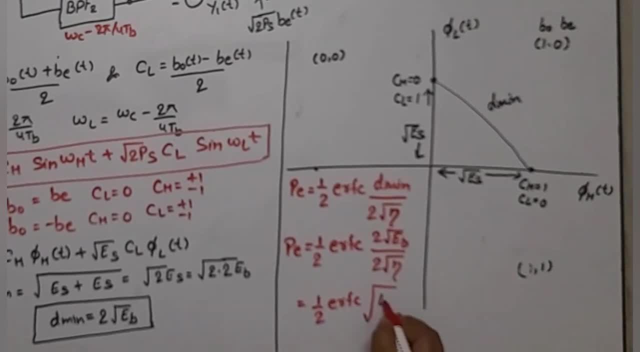 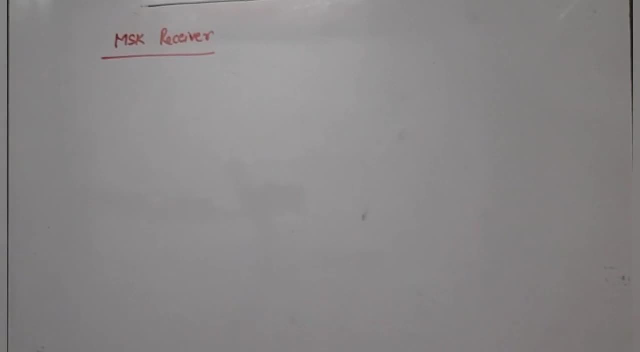 probability of error for MSK. Okay Now MSK receiver. MSK receiver means that in this case, we receive the signal and we recover or reconstruct the original signal, message, signal which was transmitted. What the input sign here will be Here, our input sign here: 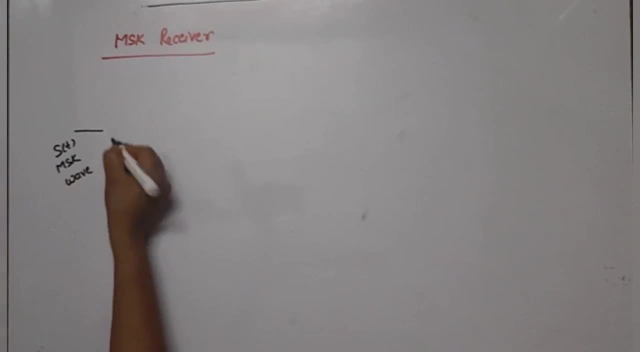 will be. ST means that this is the MSK wave. Okay, This we received. Now, when we have received it, we will apply it to весь, to the product modulator: First produce modulator, Again, the first product modulator. So here we have our data Now. the output is 6 beefs. 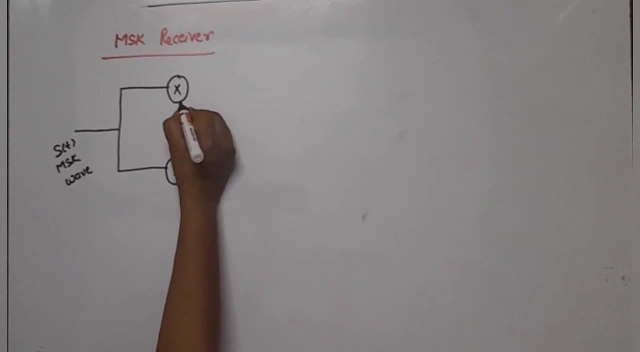 product modulator and second product modulator. okay, here our basis function will be phi ht and here what will be phi lt. okay, after this product modulator, we will pass these signals to low pass filter means to the integrator, and this integration we will do for 2 tb time. 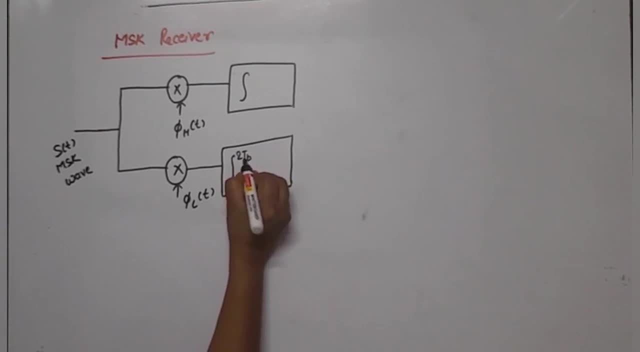 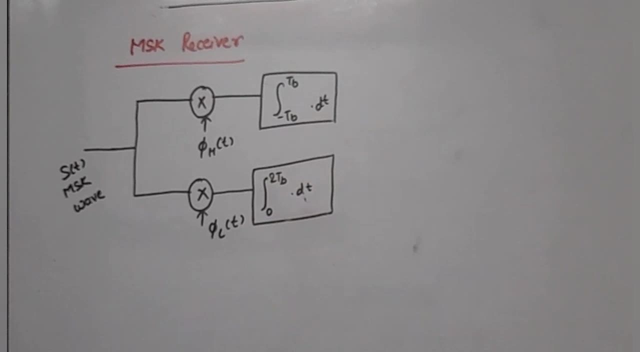 means suppose here integration will be 0 to 2 tb time, okay, and here integration will be like: this is from minus tb to tb, so our total will be 2 tb. okay, then output of this low pass filter output will be: it will block carrier signal, means it will block the omega c component. 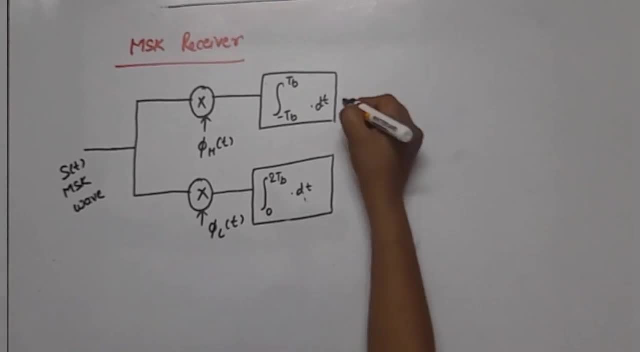 and will pass low frequency wave. now output of these low pass filter apply to decision device. now decision device will have a threshold value that is 0. here also, threshold value will be set at 0 means basically, decision device output will be like this: this is the 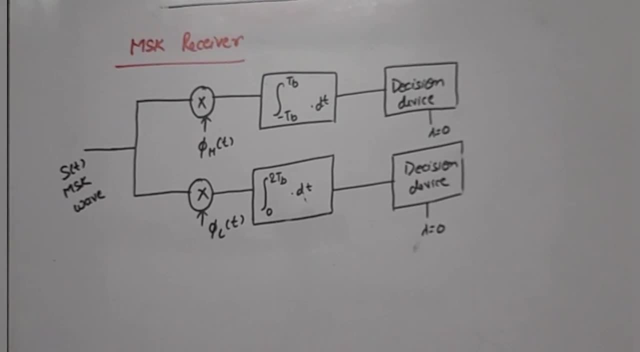 output of low pass filter, it will compare with 0. if output of low pass filter is greater than threshold value, then decision will be in favor of 1. means that what we have received, 1- 1. if output of low pass filter is less than threshold value, then this decision will be. 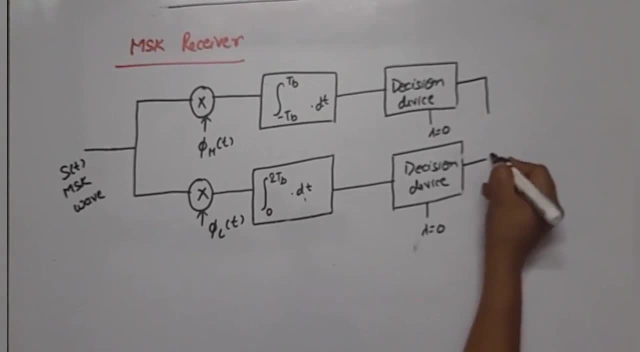 in favor of 0 means what we have received: 0. okay, of these two applied to a switch. or you can do a logic device which is inter leaving phase. okay, then output of both decision device is applied to a switch. okay, this switch will change one by one position. okay, we will keep. 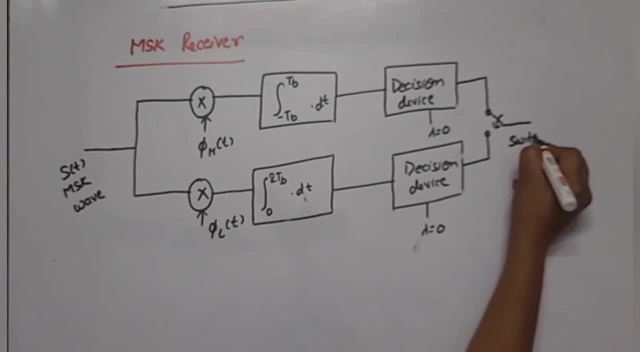 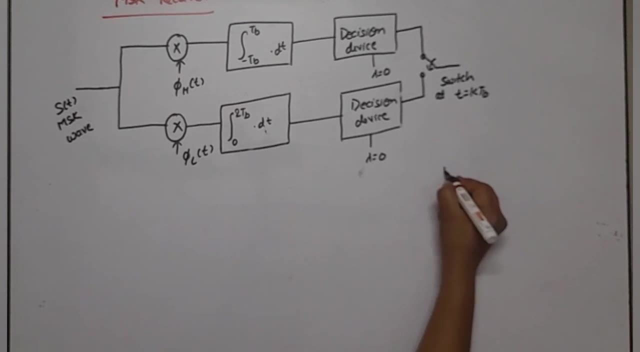 it like this: okay, So what will happen? switch at t equal to ktb. okay, so this bandwidth of msk when we draw its frequency spectrum, so the mean lobe for msk that is more than the qpsk. if we draw qpsk, then something like this happens in qpsk. okay, this happens in qpsk on our fb by 2 here: 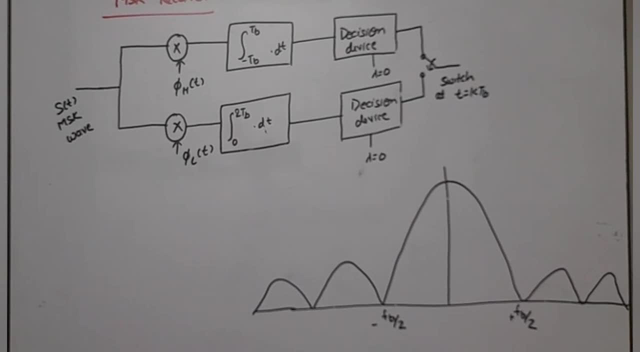 is fb by 2, this is minus, this is plus. okay, Okay, But in case of msk, what we have made it qpsk, okay. so mean lobe of msk is great, more than the qpsk. so where will it be here? okay. now what will happen? its bandwidth will increase. 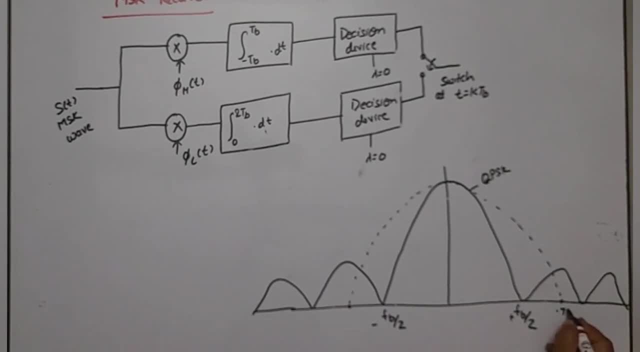 what will happen? 0.75 fb? because here it was 0.5, now its half will increase more. so what will happen? 0.75 fb? same way here, 0.75 fb with minus. so now, what is the bandwidth? this will be its bandwidth, okay. 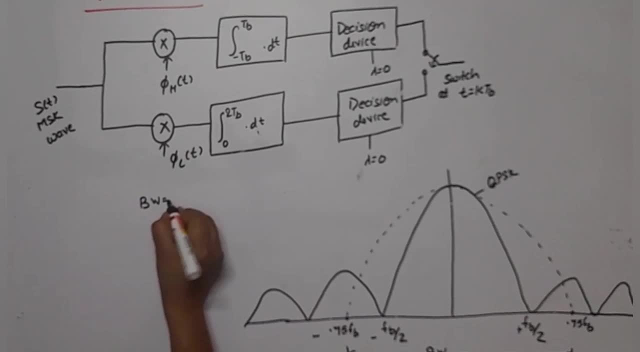 So bandwidth will be 0.75 fb. Okay, So what will happen? bandwidth is equal to 0.75 fb minus minus 0.75 fb is equal to 1.5 fb. okay, this is the bandwidth of msk. remember mean lobe of msk is greater than qpsk. okay. 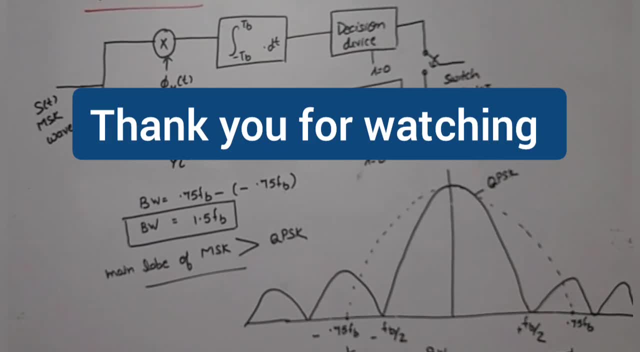 This is all about minimum shift keying. if you have any doubt at any point, please write down in comment section. Thank you. 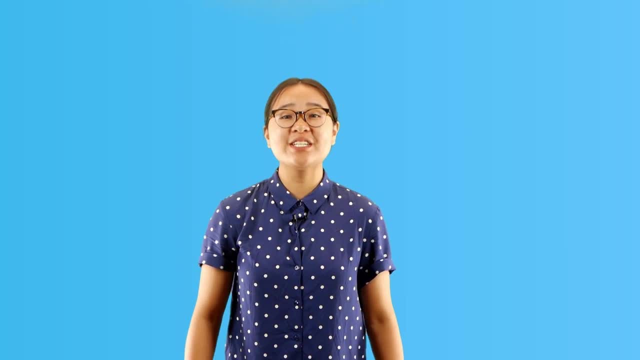 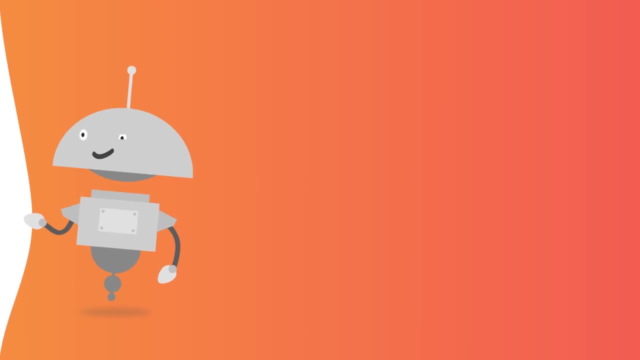 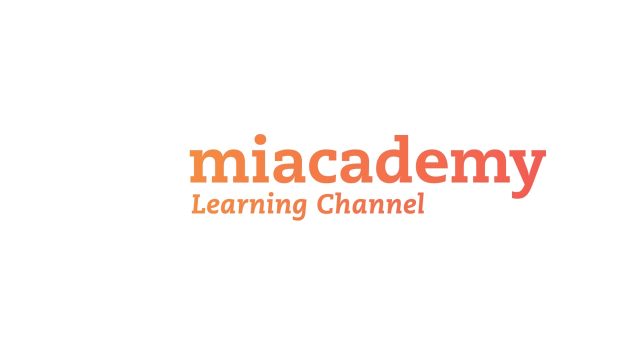 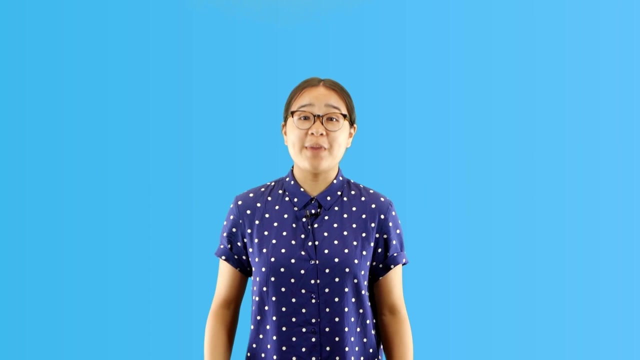 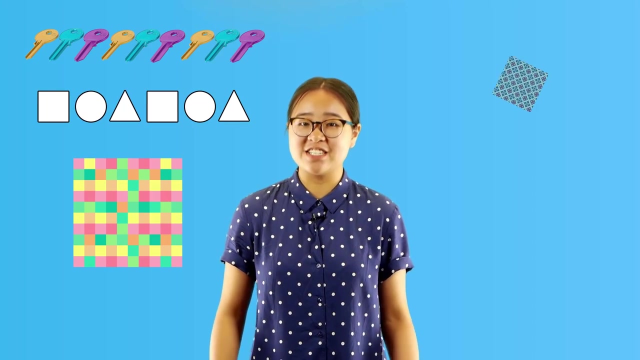 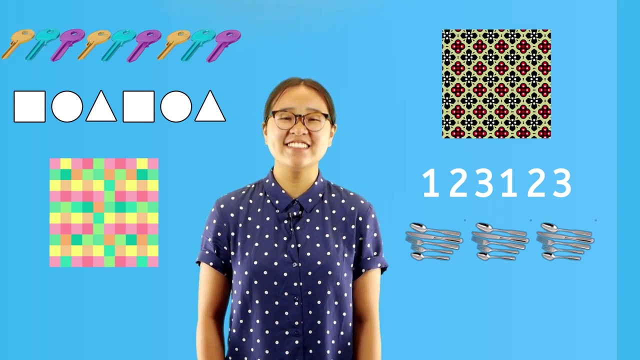 Hello and welcome to Number Sequencing. In this video you'll learn how to predict which number comes next in a series of numbers. Patterns are all around us. Patterns can be repeated items, shapes, colors, images or numbers. Sometimes a set of things are repeated to create a pattern. 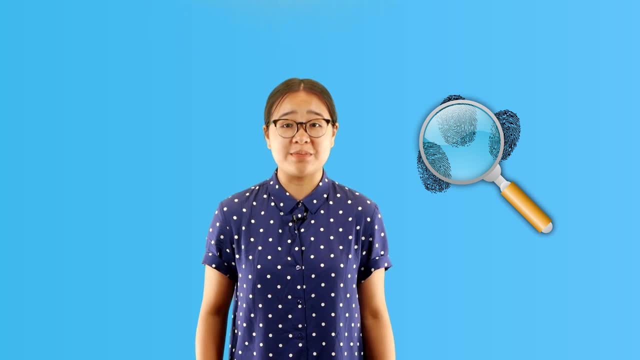 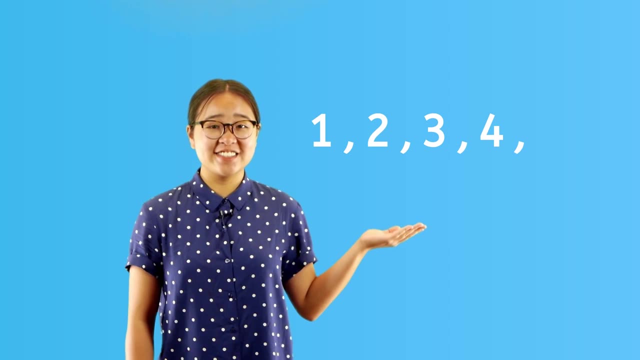 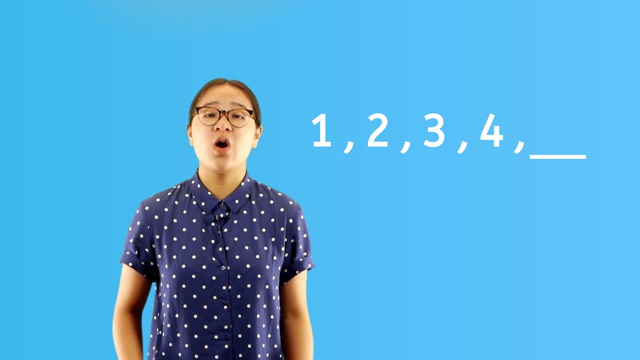 Number patterns are fun because you need to look carefully for clues to complete them. Here is a number pattern, or a sequence of numbers. What comes next? This is a fairly easy pattern because we count this one all the time: 1., 2.. 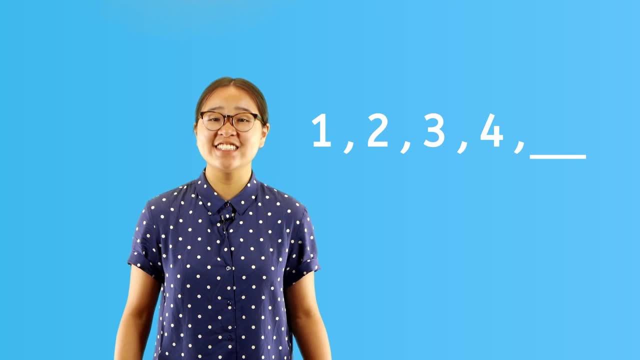 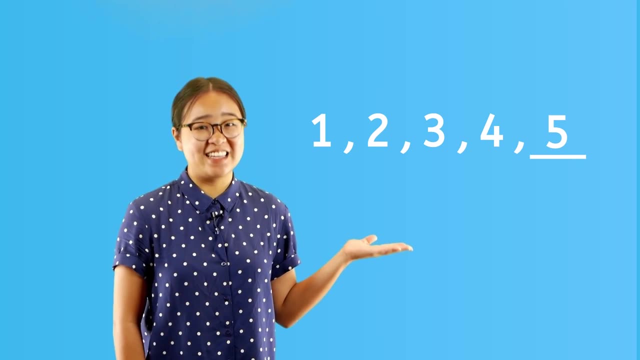 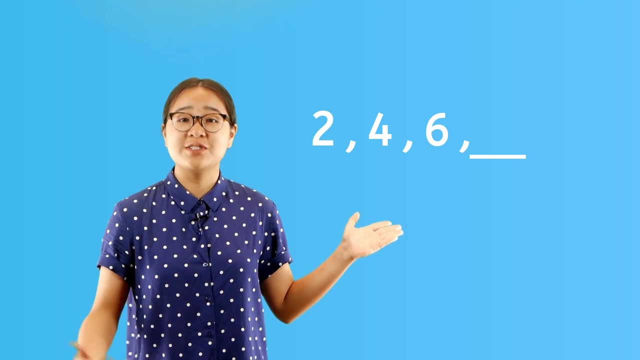 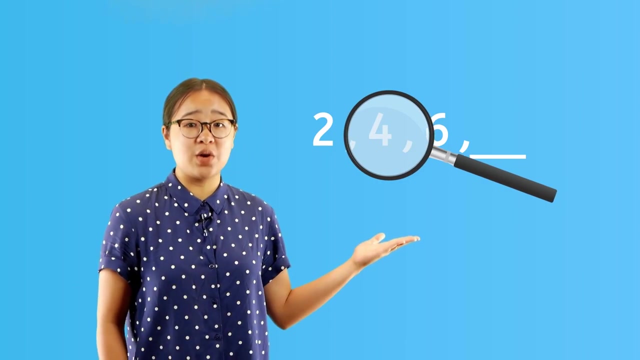 3., 4. And what comes next? Yes, 5.. Number 5 completes this pattern. Here is another one. What comes next? Let's see. We have 2,, 4,, 6. If you look for clues, we see that each number in this sequence is greater by 2.. 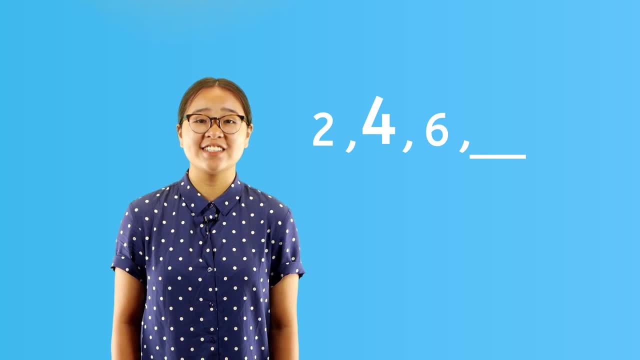 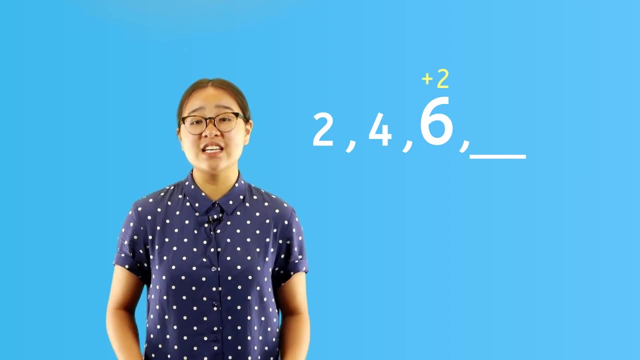